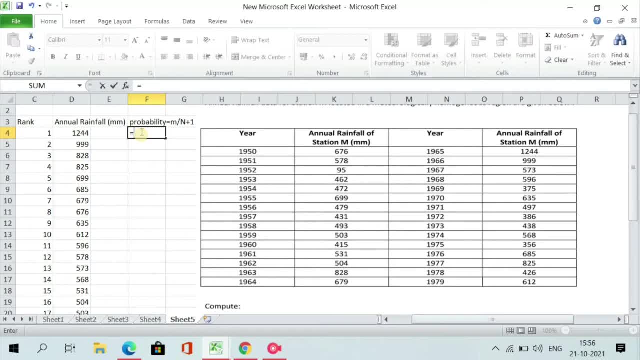 So we will be calculating probability. So first put equal to sign, Then C4. Divided by 31.. Press equal to sign, Press equal to sign. This is good, This is good. This is good, Thank you. 35 divided by 31. we don't need to put formula again and again. I have put. 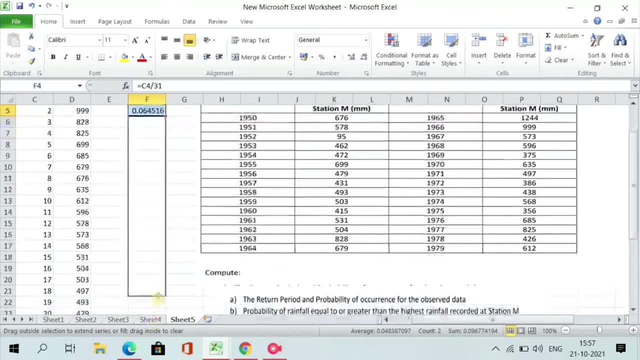 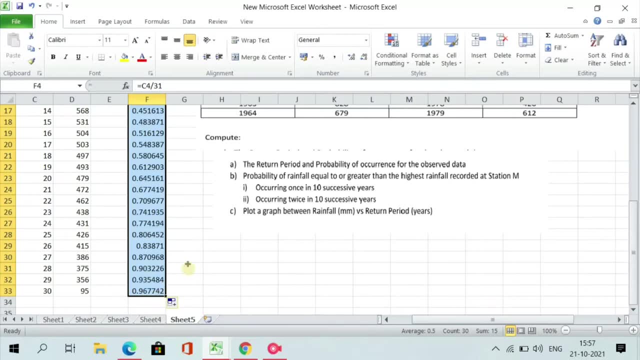 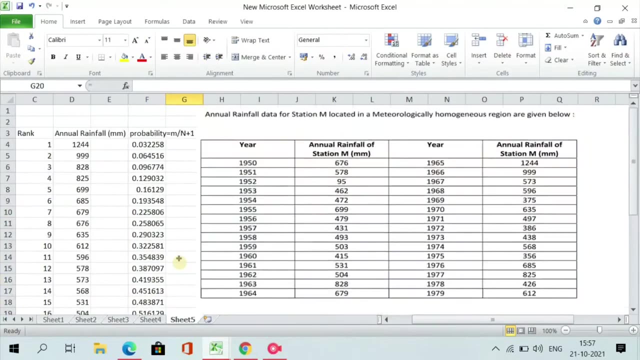 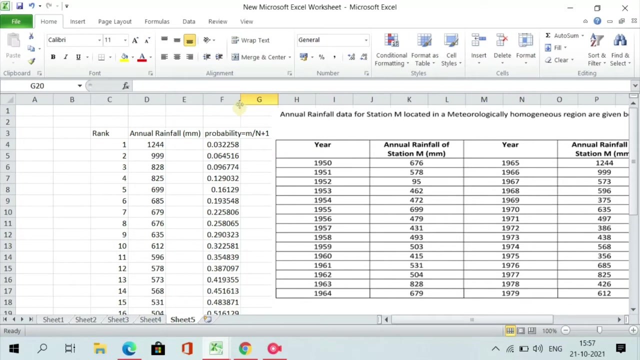 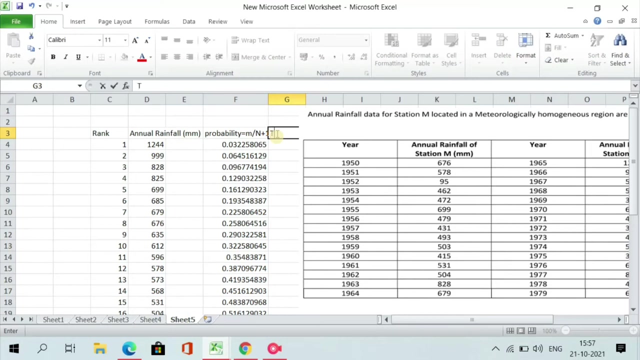 formula in two case only. I will be selecting this and this is I will be pasting. you can see we calculated the probability for all the recorded events. now I will be calculating the return period. so for the return period, for the return period, we know the formula T is equal to 1 by P, that is capital T. 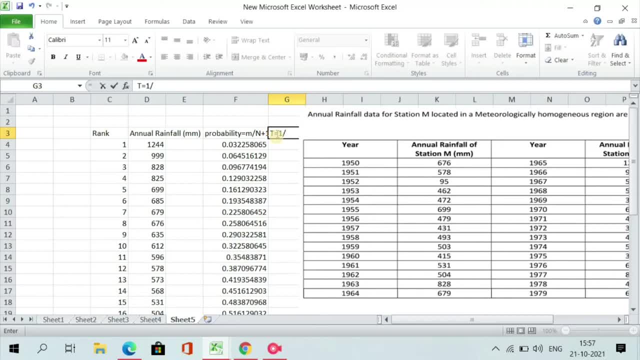 capital T is equal to 1 by P. that is capital T. capital T is equal to 1 by P. we need to do this, the reciprocal of column F. so what I will be doing- 1 by f4, put equal to sign first, 1 by f4- we need to do is: plus buzz, press enter sign 31 and press enter. 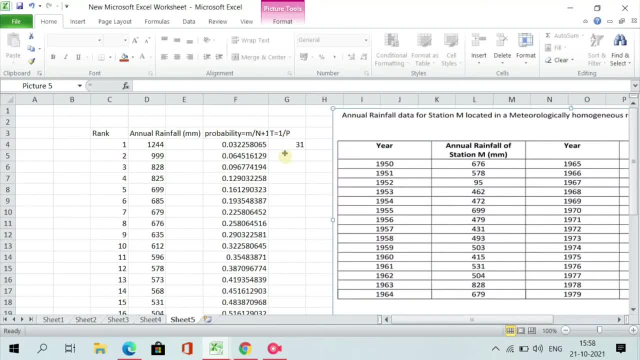 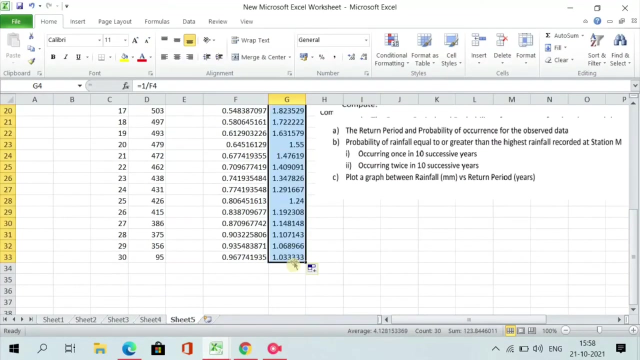 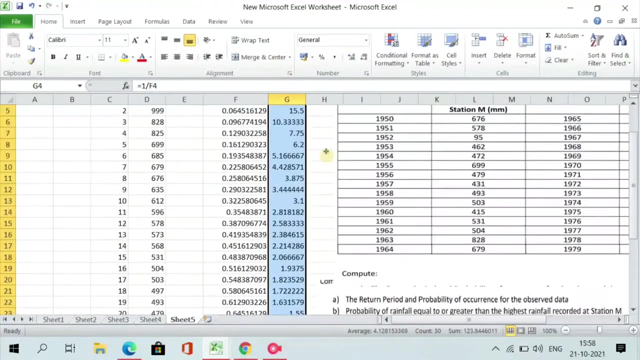 press enter sign 31 and again put formula equal to 1 by an five. again put formula equal to 1 by an five four. We don't need to put formula again and again. we will drag to get the return period for all the recorded events as we got the return period for the all recorded events. you can. 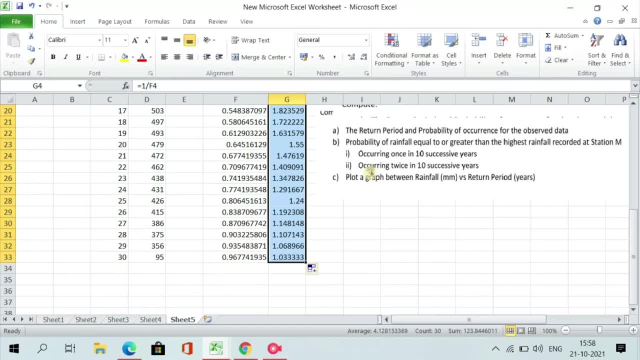 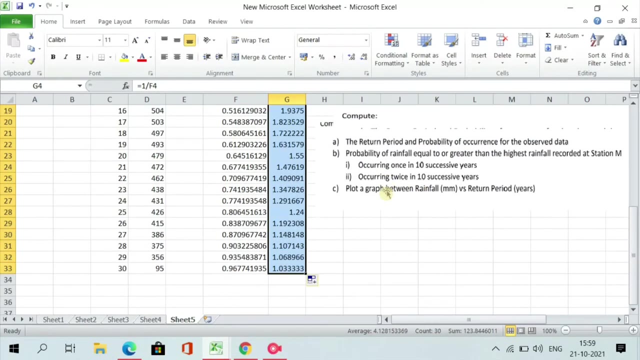 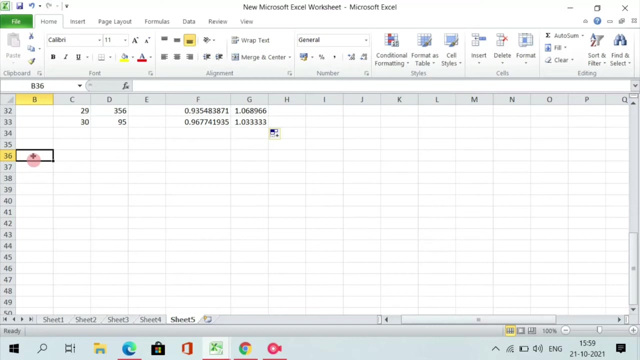 see now. so already we have completed our first problem: the return period and probability of occurrence for the observed data we have calculated. now I will be plotting a graph between rainfall and return provide. I will be solving this problem at last. V problem: first let us do C problem. so plot the graph between rainfall, individual per year. so I 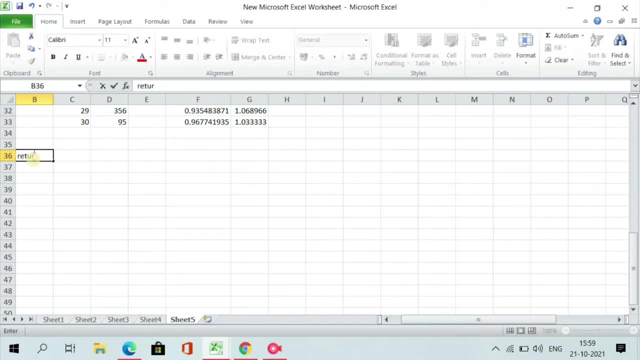 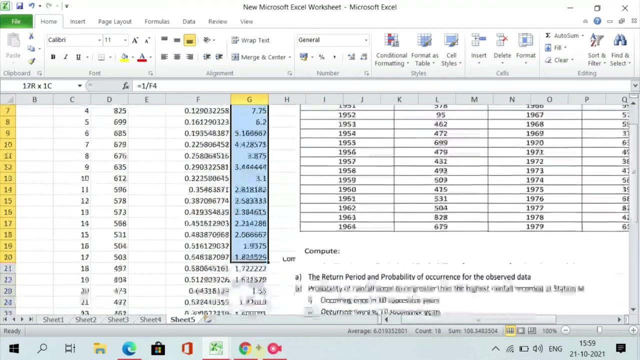 have written period. return period should be or should be on a x axis: x axis return period. we will form another table return period. we will just Copy and paste as your way. annual rent fall in mm. we have to just copy and paste return period from here. we have. 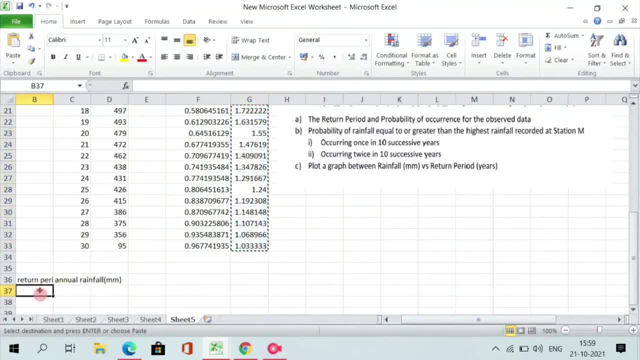 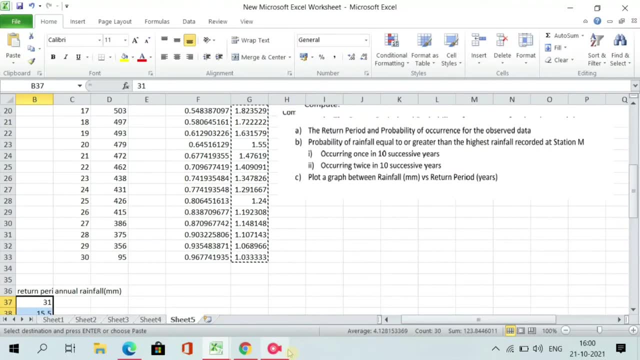 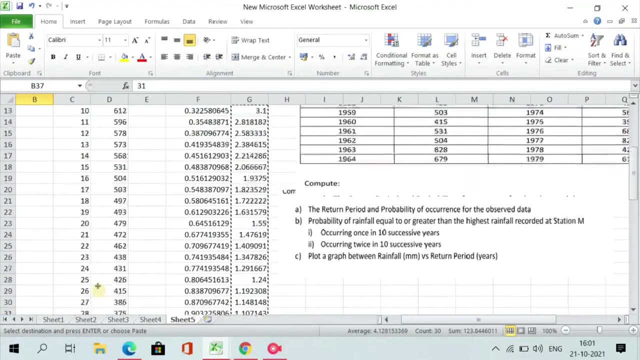 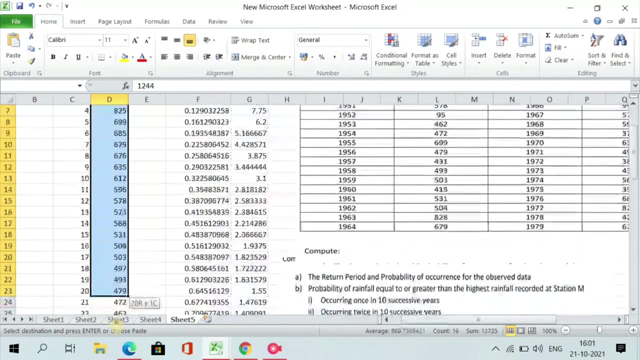 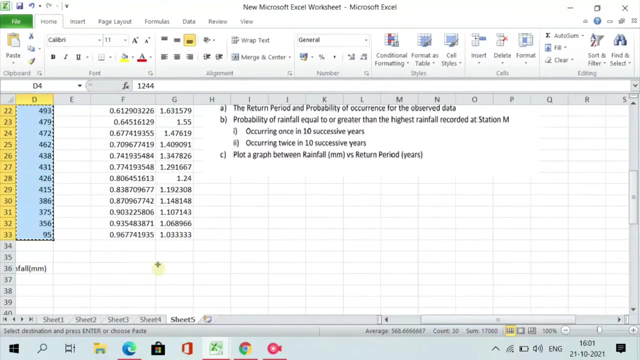 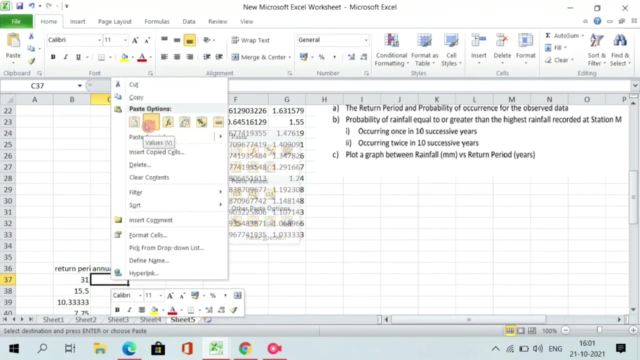 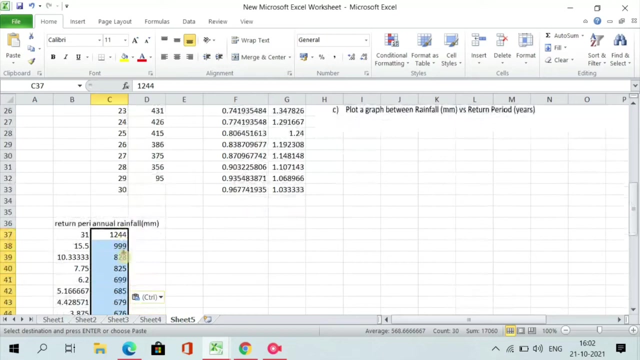 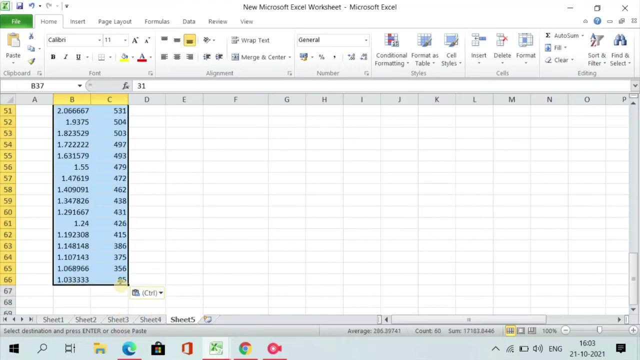 to copy, and here we will be. will be copying annual rainfall data from here. let us copy now. here we need to paste, as we have completed the table for the inserting of the graph, but we know the rent fall magnitude is floated against the corresponding table return period on a semi log paper now, so maybe we will be selecting these two data. 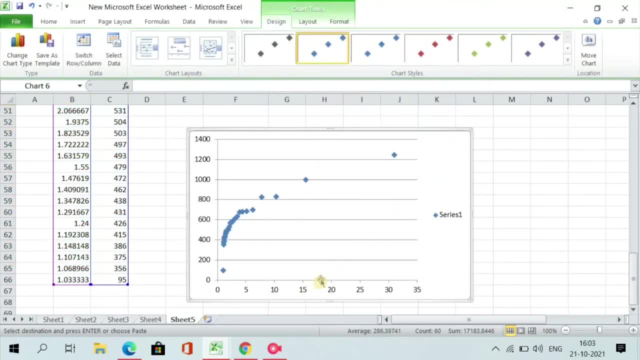 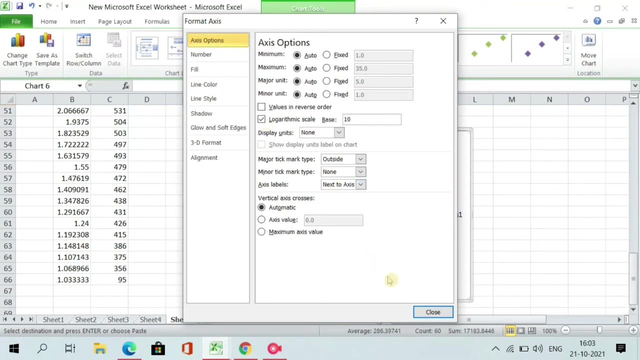 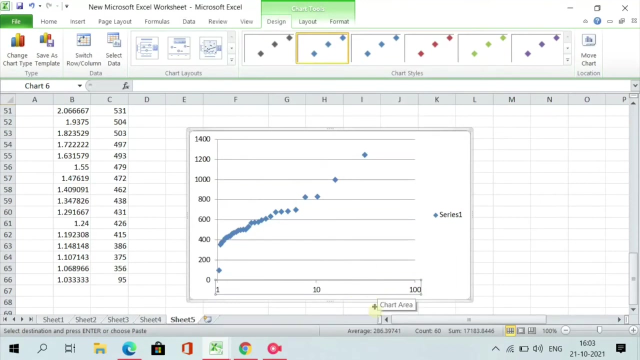 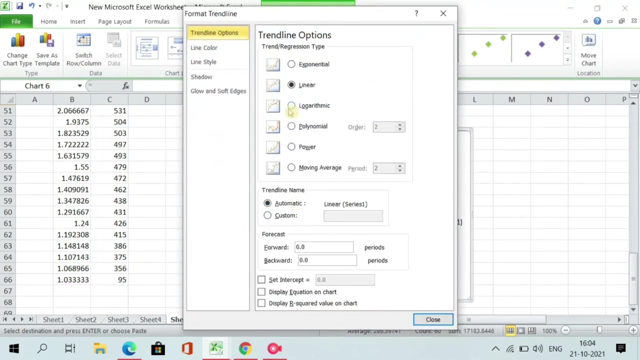 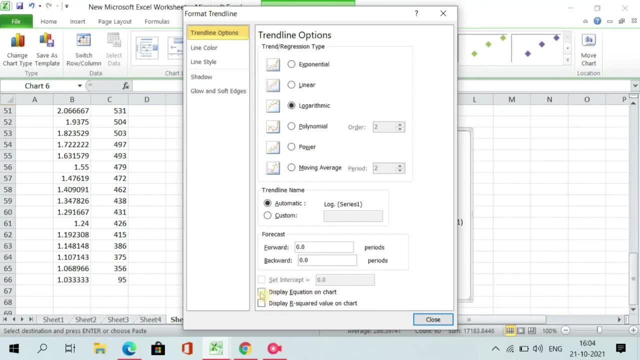 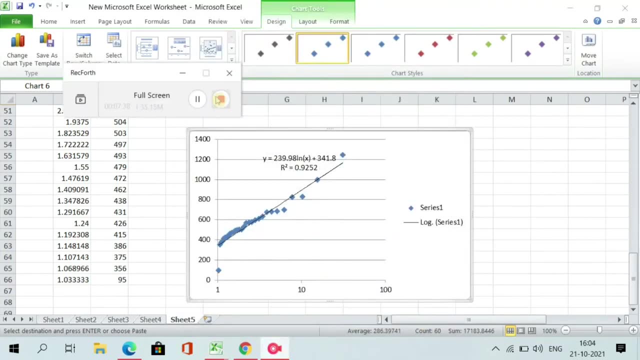 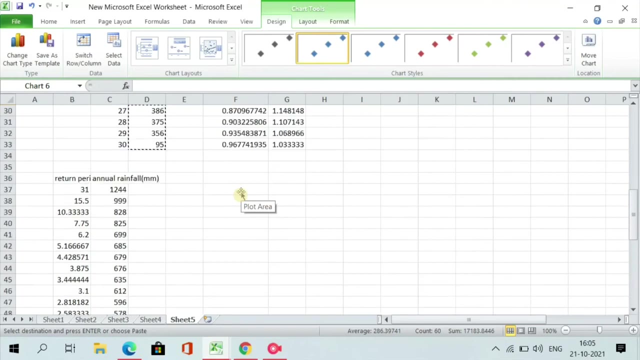 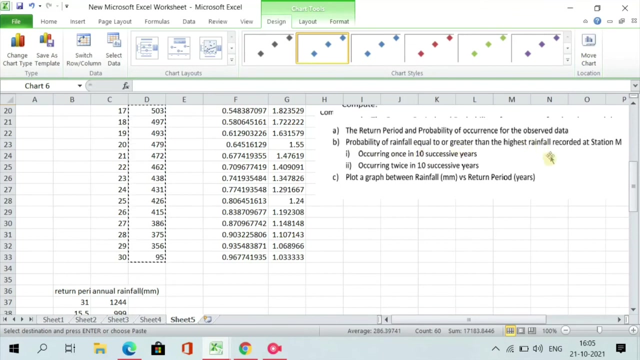 at trend line logarithmic. if we want display equation, take it. if you want display r square value on chart, take it, close it. this is our required graph. this is our required plot. we have completed c number question. also, now we will be discussing probability of rainfall equal to or greater than the highest rainfall recorded station m. we will be solving this. 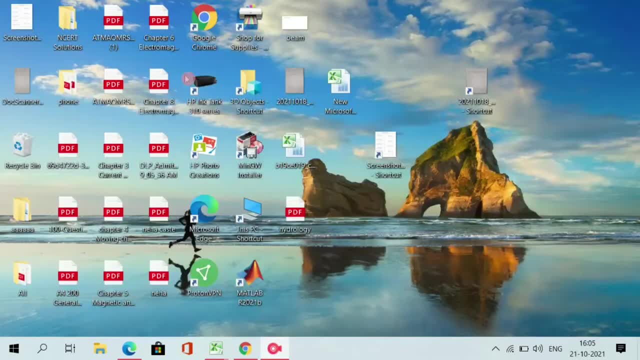 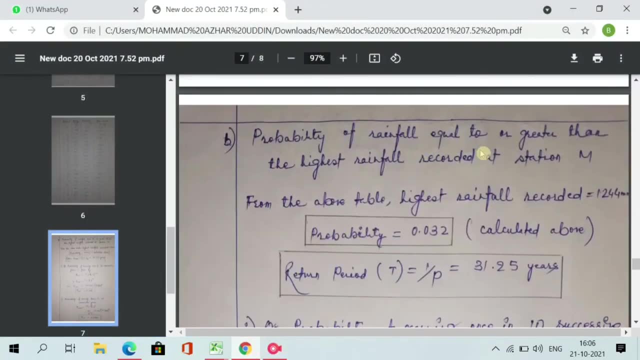 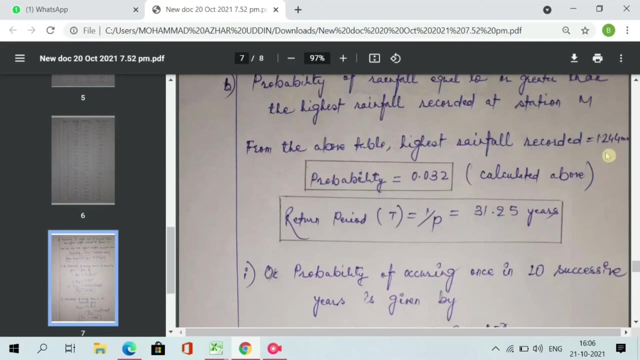 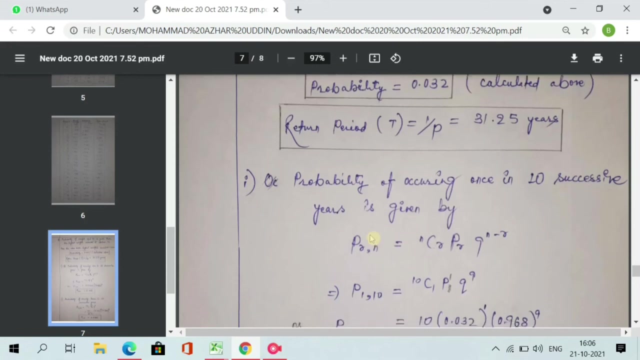 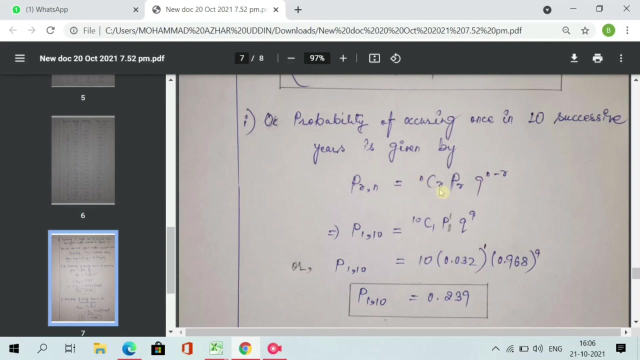 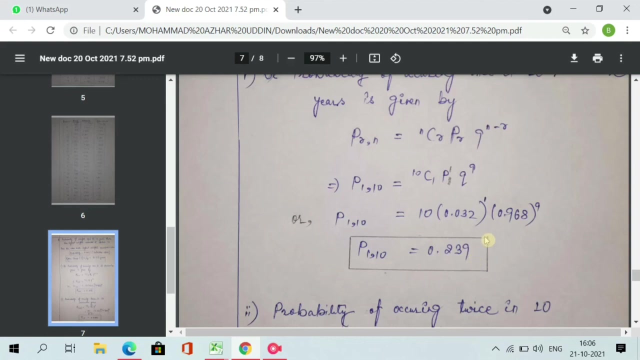 so let us see how we are solving this. so probability of rainfall equal to or greater than the highest rainfall recorded, station m from the above table, the highest rainfall recorded is equal to 1244, as we have already seen there, um and q is non-occurrence of the event. so after substituting, we got the, we got this, this, this.